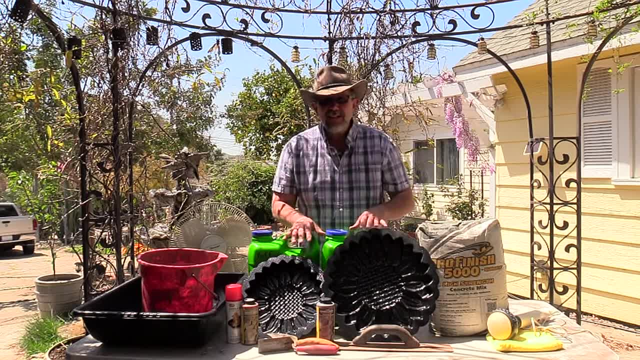 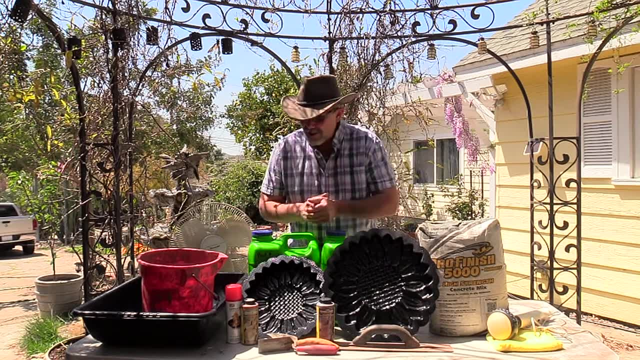 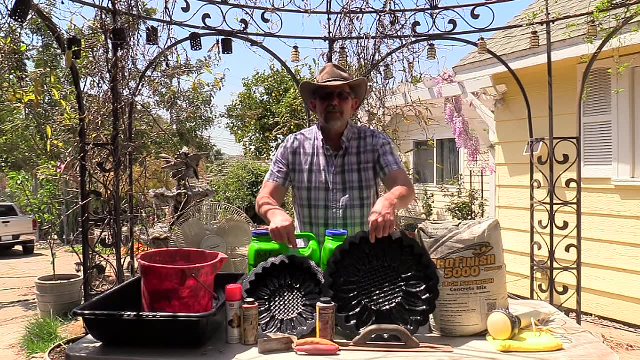 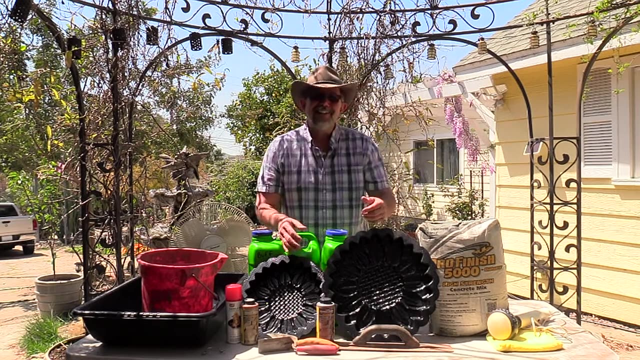 to be putting into these. If you're new at casting concrete, you know. watch the whole video. I'm going to go step by step by step, showing you all the steps that I take for this, And I'll be using all of this stuff And you'll see how it's being used. So come on along And let's make some decorative stepping stones or decorative yard art, which I'm going to be using it for in my garden. Okay, come on along. Okay, so the first thing I'm going to do is 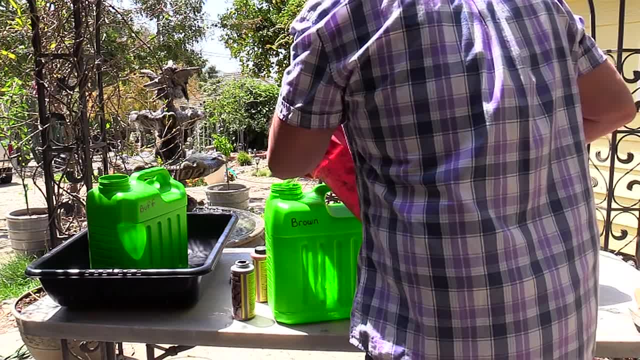 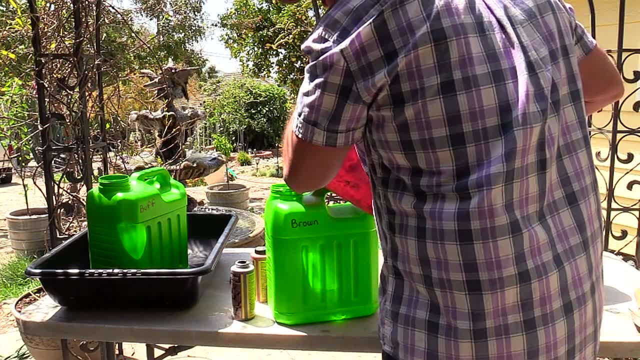 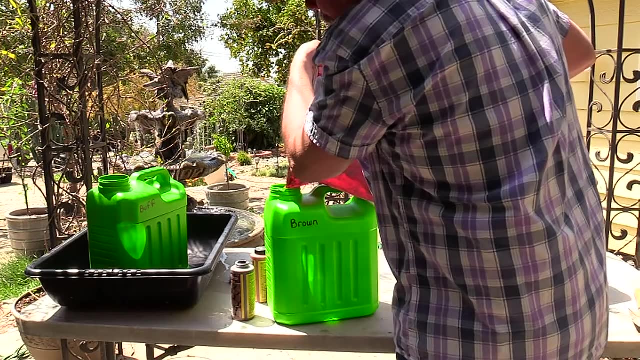 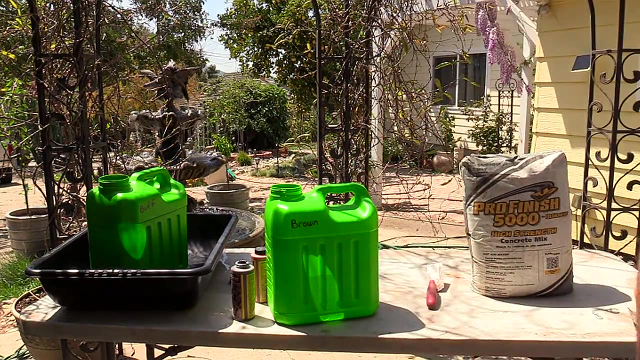 add a gallon and a half of water for the brown. You know, for the brown, technically you could get away with three gallons of water, But I want the brown to be really strong or very pronounced. So I'm going- you know basically what- you would mix one bag with one bag of concrete. So I've got my water in And now I'm going to pour this. So you be careful with it. This is really really. 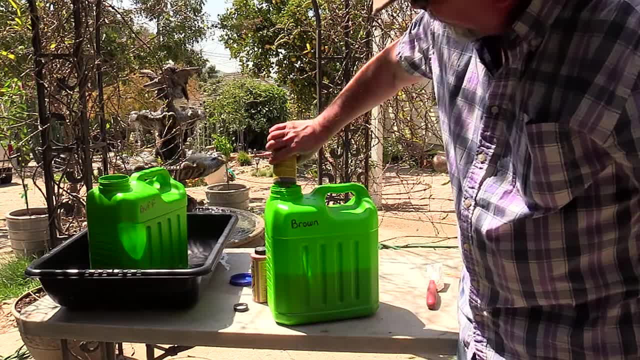 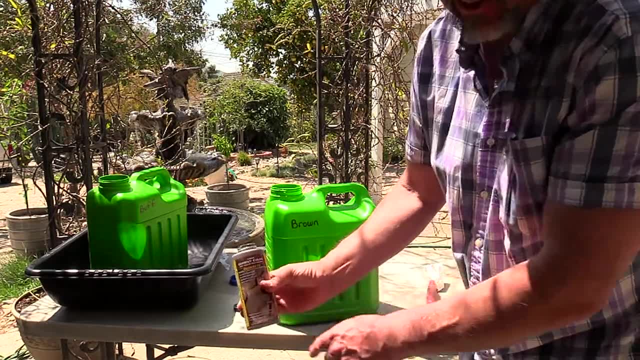 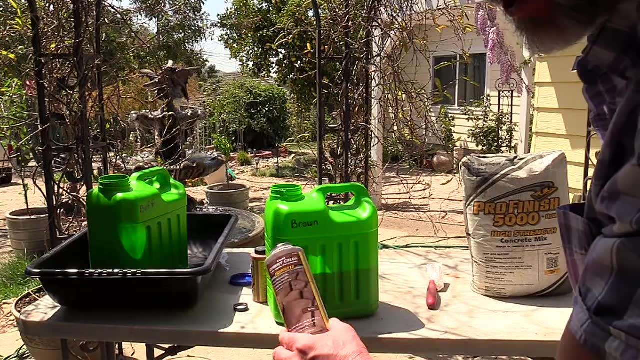 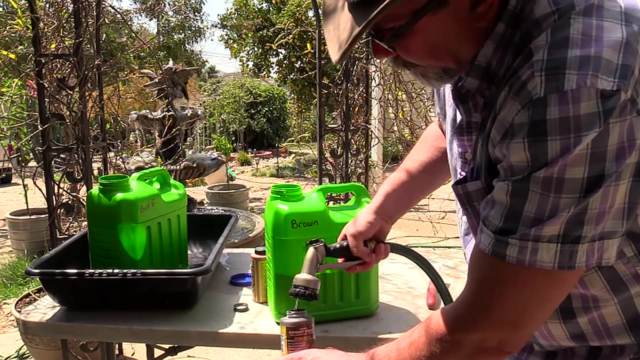 messy. So, as much as you can, try not to spill it Now with the brown there's every bottle. there's going to be leftover colorant in here, So what you want to do is to put water in here, put the lid back on and shake it up to clear out the bottle. So you stay consistent. I'm going to go ahead and add water. you know enough to help clear this bottle out. Once again, to stay clean, put that lid on nice and tight. 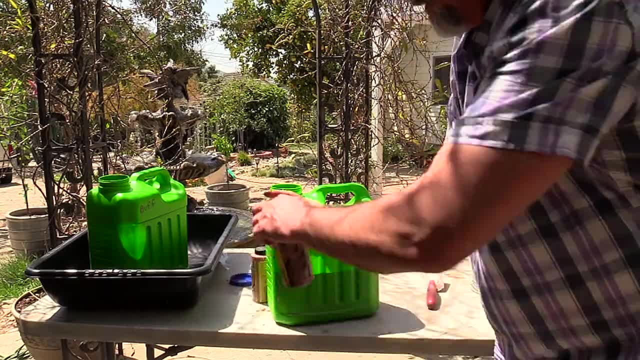 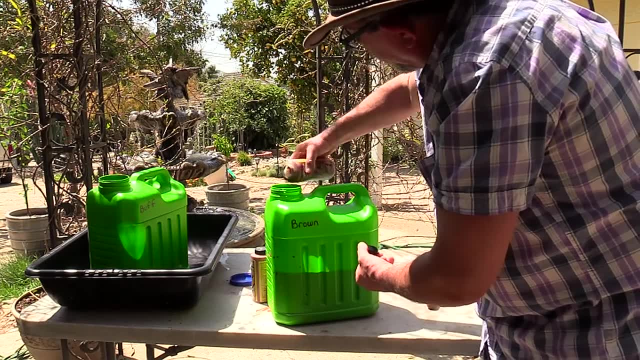 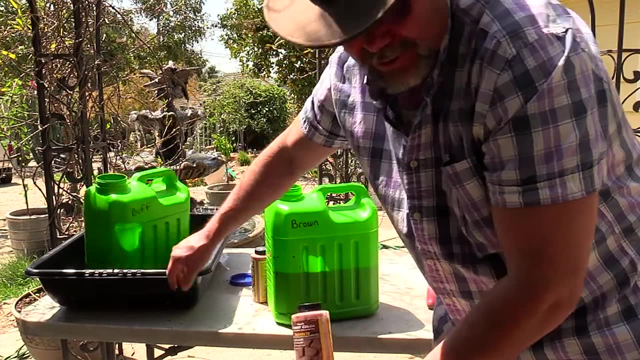 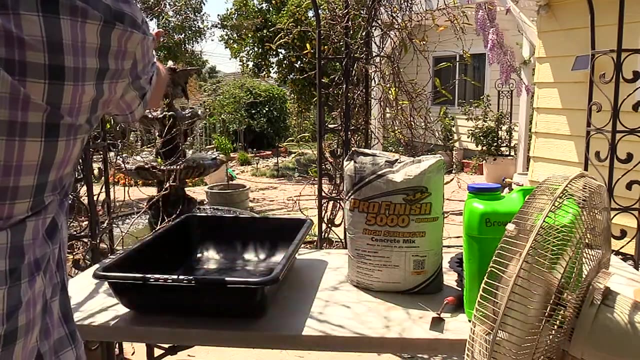 And shake it up And we'll go ahead and pour that in And we're looking real good And I'm taking it to about a gallon and a half. This will be about three gallons the buck. Okay, so you can see I have a fan going That's to blow or move the concrete dust in that direction. You notice that the fan is blowing it in the opposite direction. 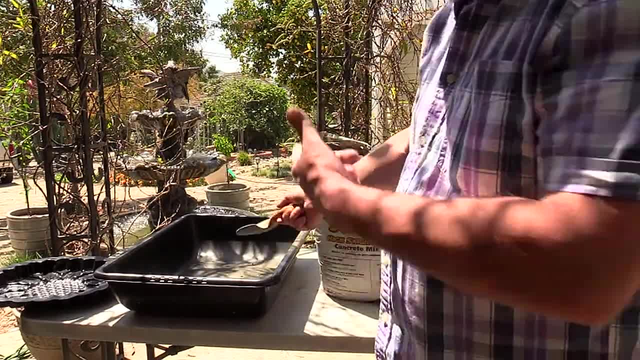 Okay, so you can see, I have a fan going That's to blow or move the concrete dust in that direction. You notice that the fan is blowing it in the opposite direction. You notice that the fan is blowing it in the opposite direction. You don't want to breathe this. You know, if you don't have a fan, use a respirator. 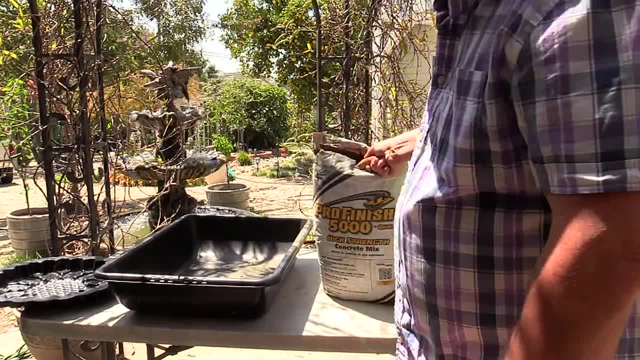 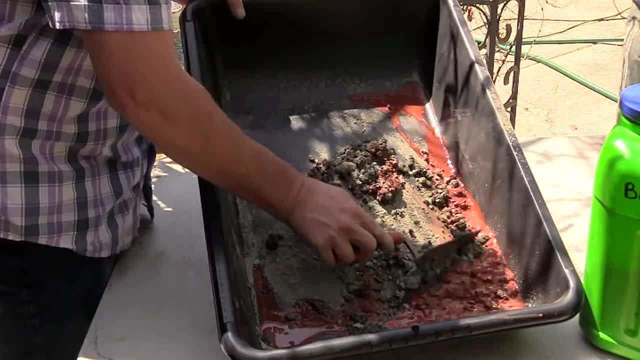 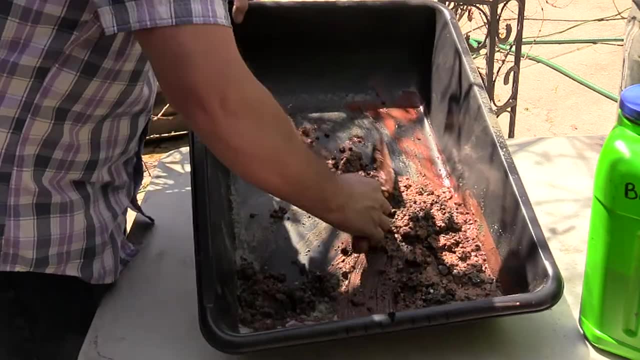 And also wear. you know some kind of goggles, But eyeball the water pouring, You know, go very strongly, You can always add more. And also wear. you know some kind of goggles, But eyeball the water pouring, You know, go very strongly, You can always add more. 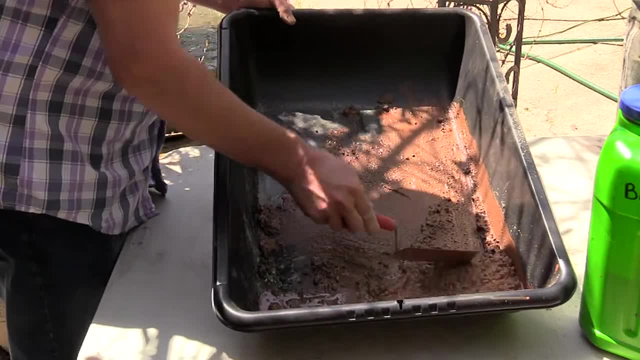 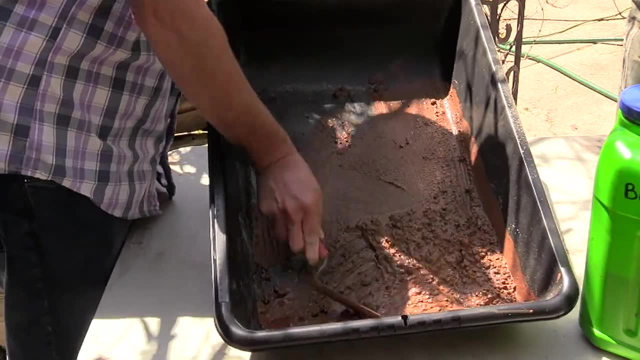 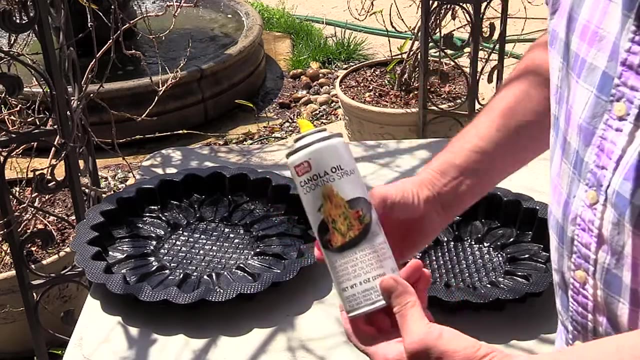 This is a good consistency for me. Real nice mix Color seems to be in there pretty well. There's a little gray I need to get rid of. Next step is prepare the mold. Okay, so, concrete's a very sticky thing and you want something to release it. 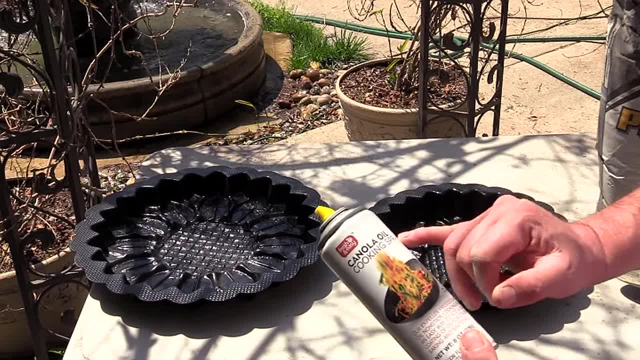 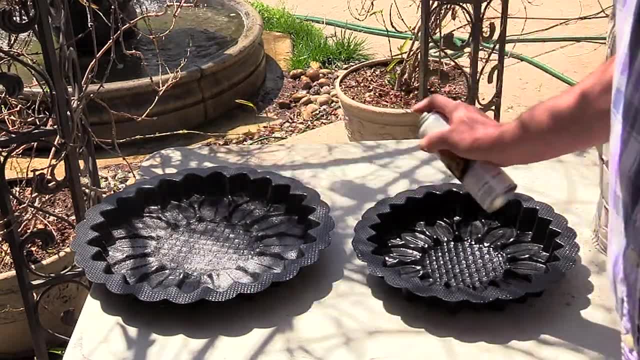 I'm going to use something natural: cooking oil spray. You know you could use motor oil, but who wants to get motor oil on their hand? I'm just going to give it a light spray and then I'll wipe it with a rag. 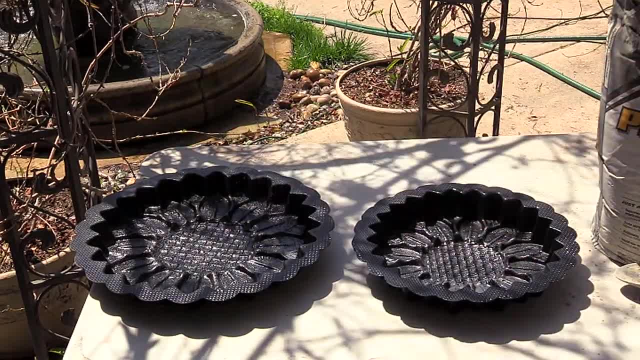 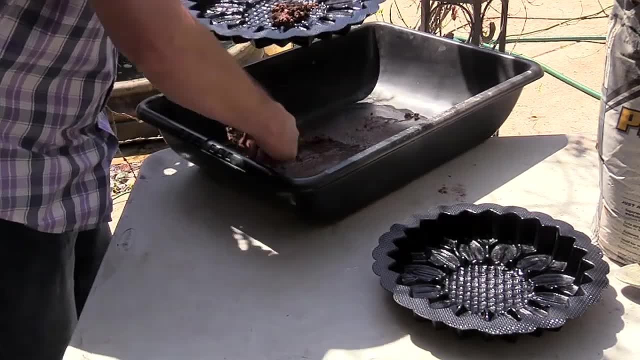 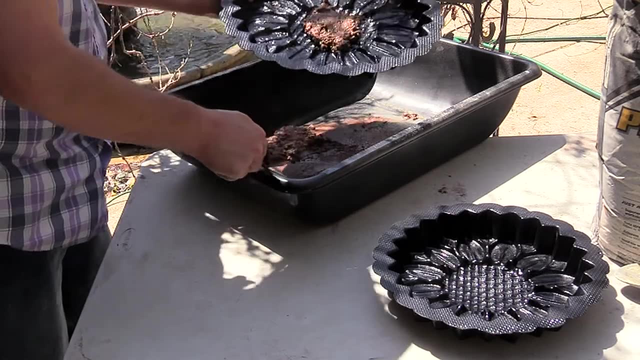 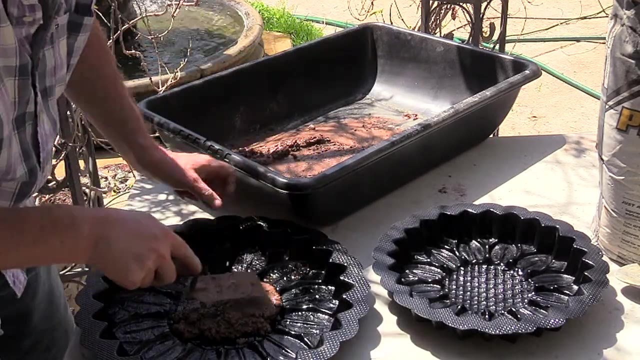 And that looks real good to me. Put in my brown Shovel it in there. There we go. Make sure you can see that I'm putting it in. I'm going to go a little bit high, But I want to stay out where the flowers are, so I'm going to come up high and then, at an angle, 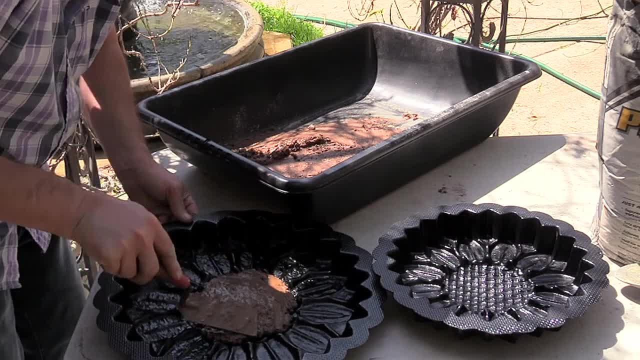 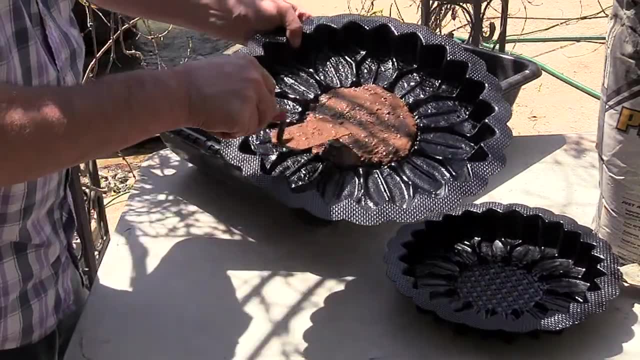 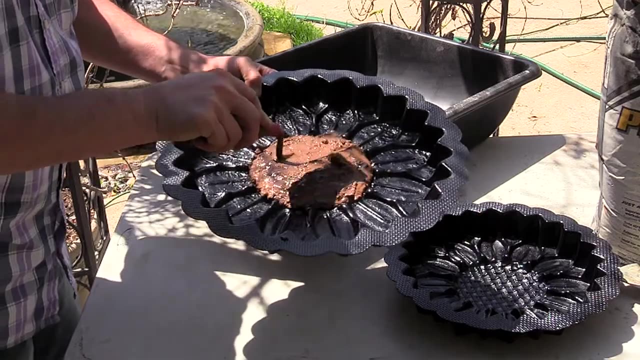 Like this: Let it sit high up here And then I can work it down and around there. Hope you can see that what I'm doing. Try and hold this up. They sell professional table vibrators for this kind of work, But you know, I've found that using a general muscle massager works really well. 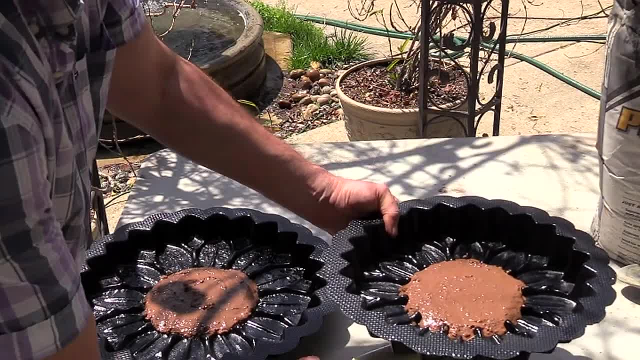 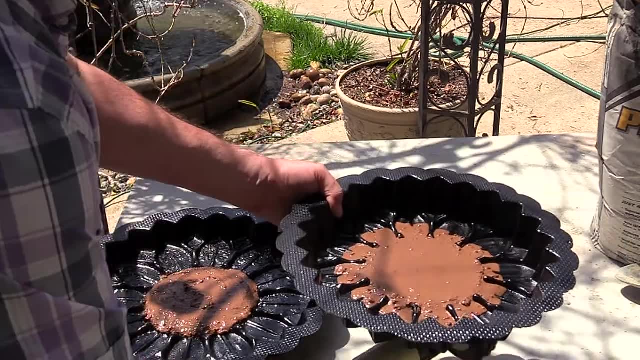 You want to get the air bubbles out And you can see that the cement's going to run out. I'll push it back, But it's going to help get rid of these bubbles. You can see the bubbles coming up And I'll come back and clean it up in a minute. 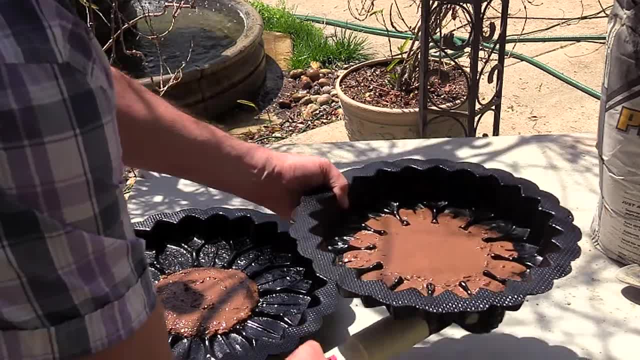 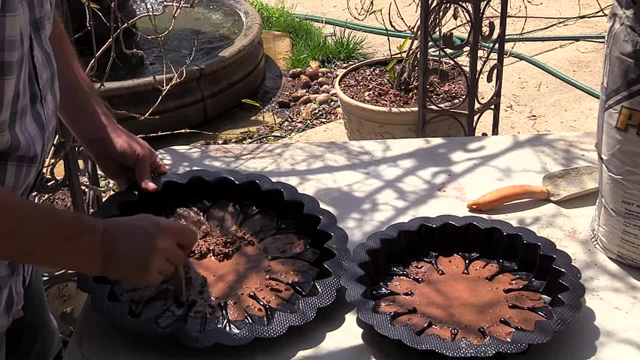 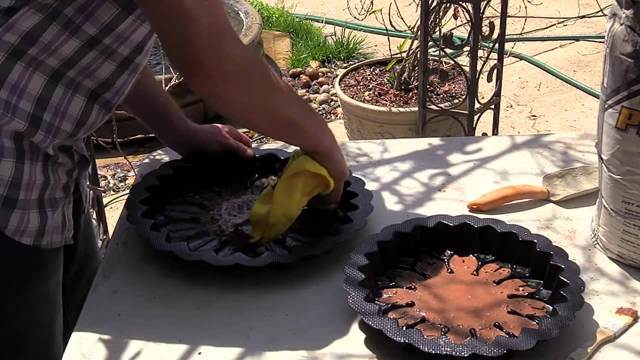 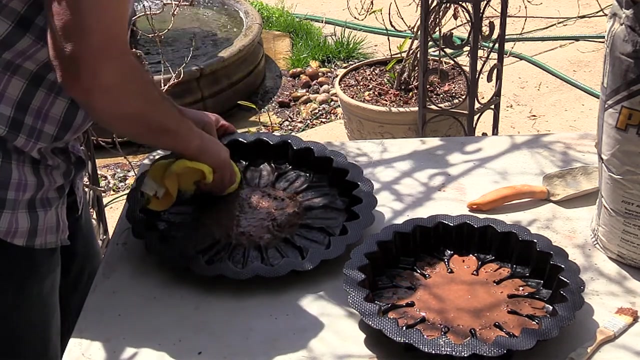 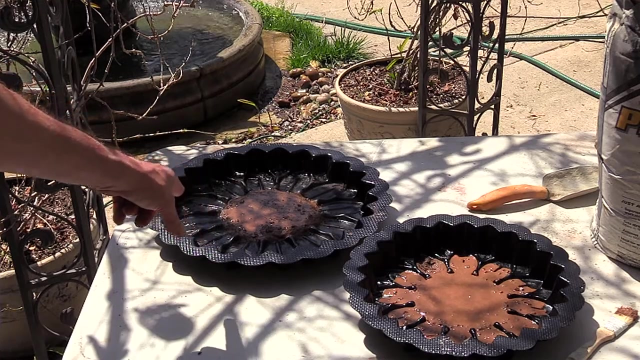 And you can see the bubbles popping up And that will kind of affect your casting. Push them back to the bowl And then I'll come back with a rag and wipe it to get the brown out of there. I will be pouring in buff after about two hours is what I'm going to wait for this? 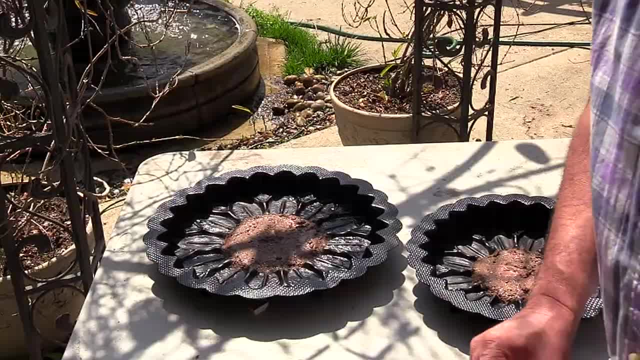 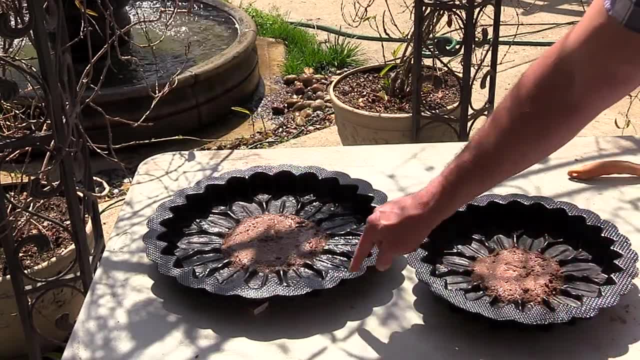 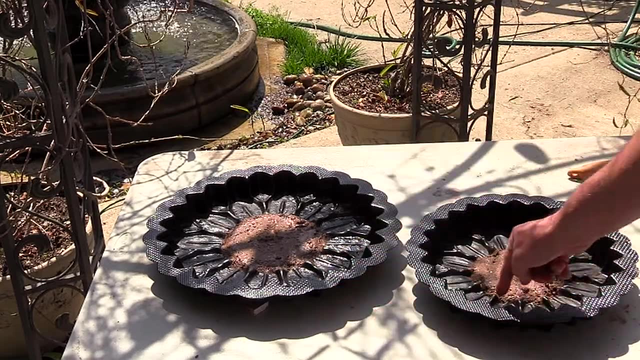 Two hours for this to start solidifying. Okay, so I'm getting ready for the pour. I made these risers. They're about three-eighths of an inch high Because the seed component on this particular casting is lower than the floral part. 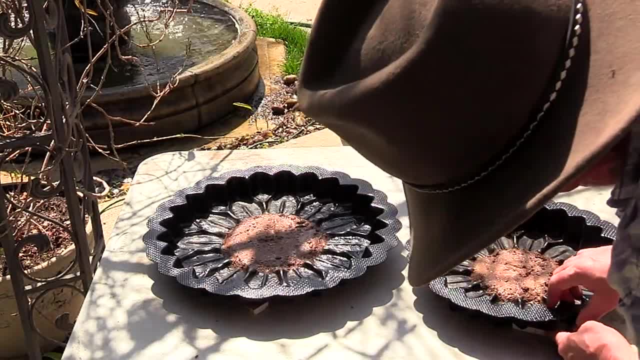 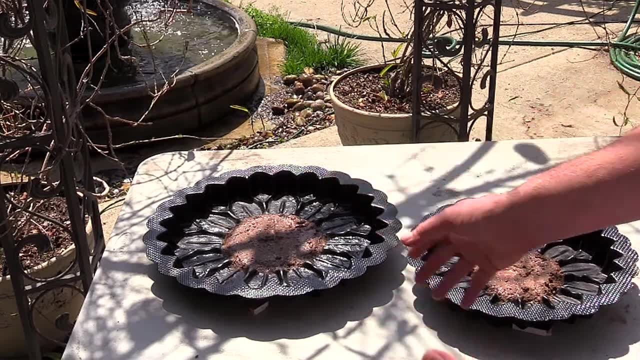 So I'm putting them under here to hold it up, to keep everything. even You could easily, you know, put them in a box of sand to cast it if you wanted to, But I'm going to go ahead and use this technique. You can see I've got them here staying off of the concrete here. 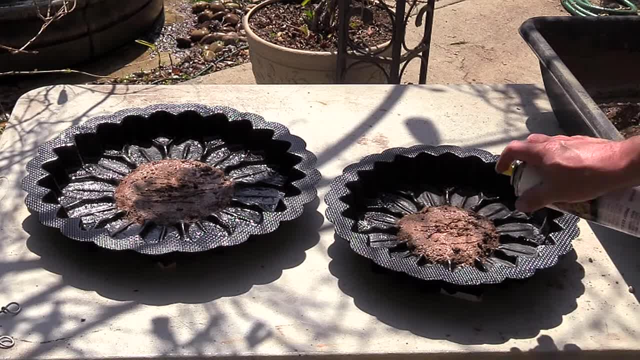 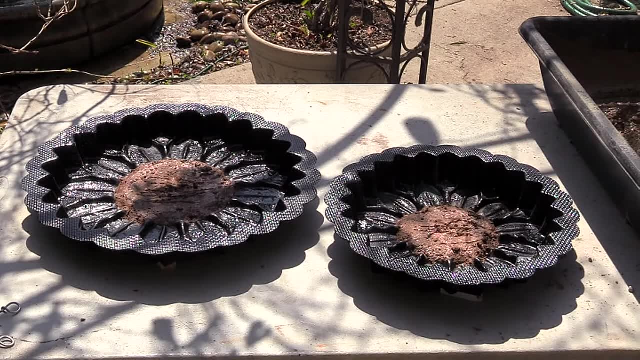 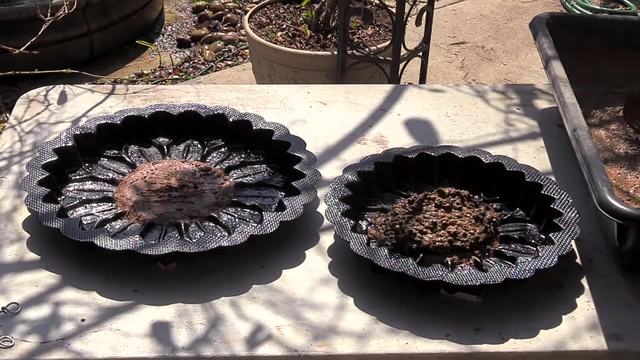 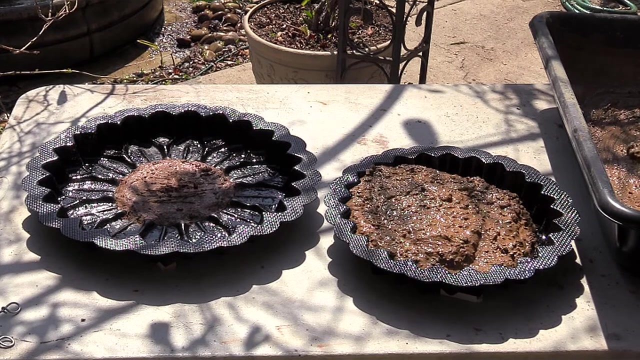 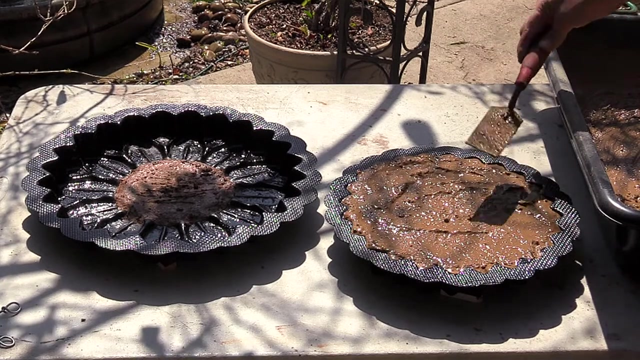 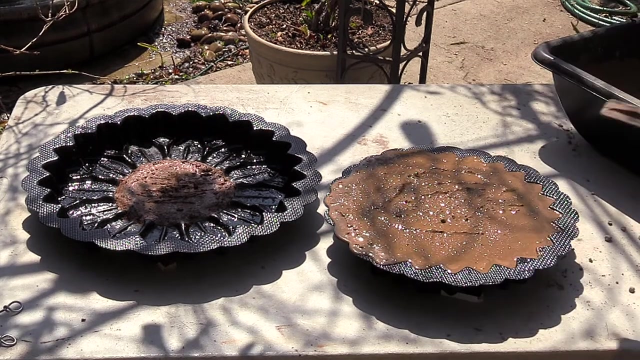 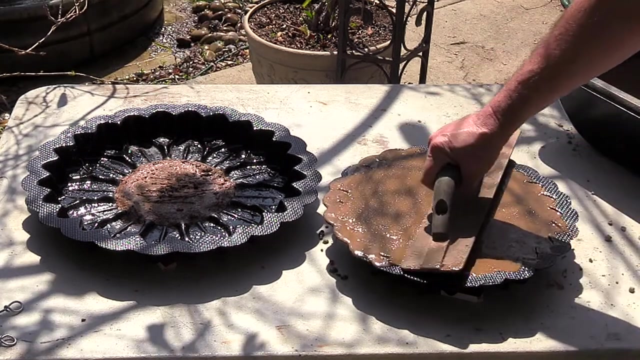 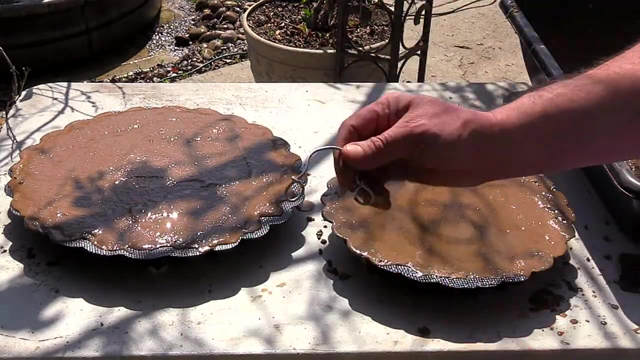 There's no reason to get oil on that. You want those two to stick together nicely, which they should do, just fine, And there we go. okay, so it's pretty much done. you know I'm not going to put this in, but you're going to use. 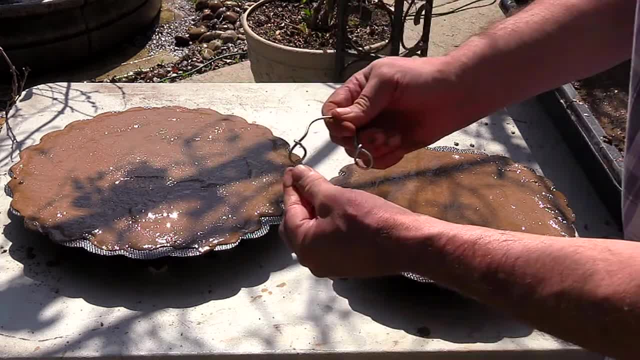 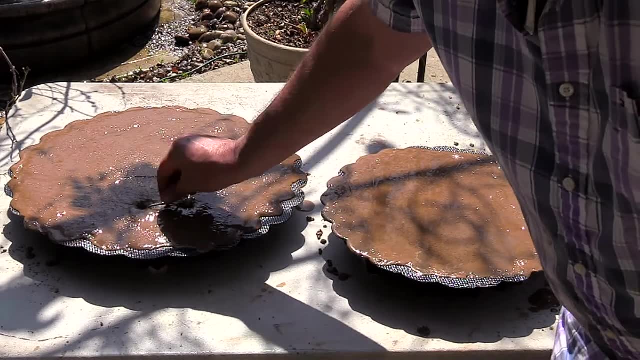 these, as some people like to hang things on their garden walls. notice that it's got its loops and it's wired here. so you'd be slip it into the concrete. I'll go ahead and do it and remove it. you slip it down in here like that, work it in and those loops, the concrete would. 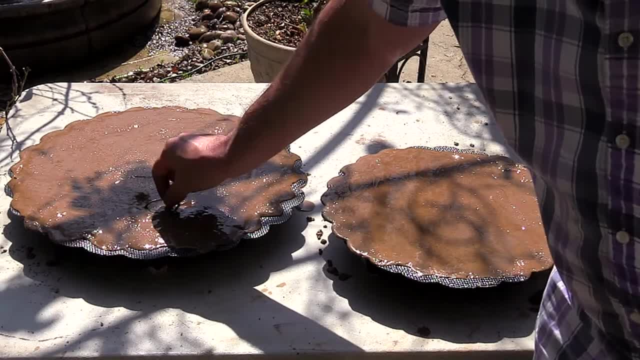 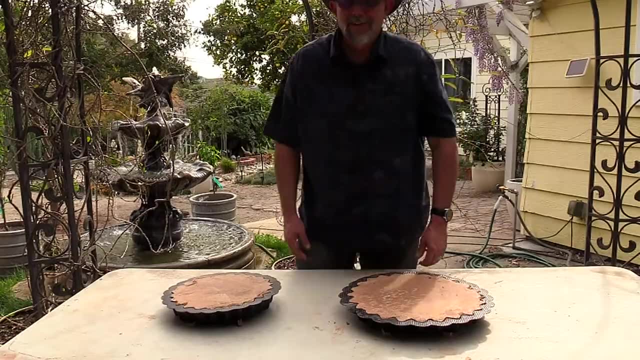 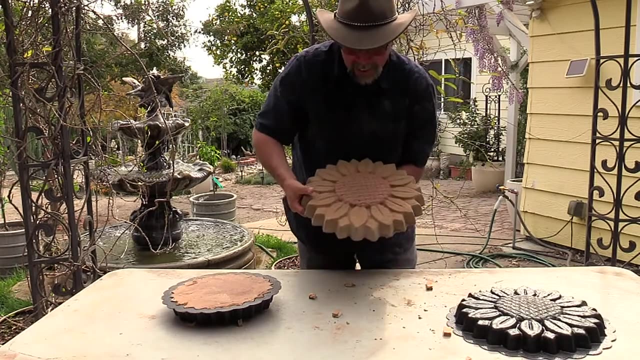 come around and surround it and it wouldn't come out and you could use it for a hanger. I'm gonna- I'm not going to, I just wanted to show that to you, so tomorrow I'll remove it and show you the end result. okay, so I just took these out. 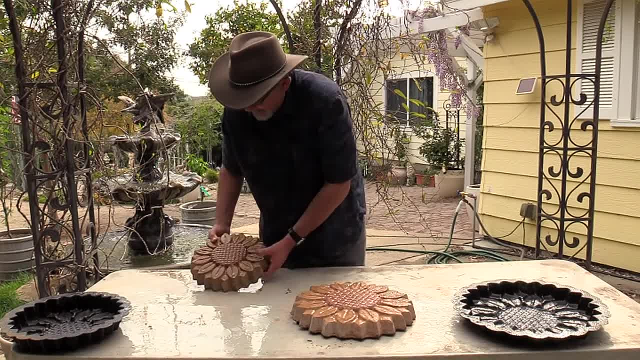 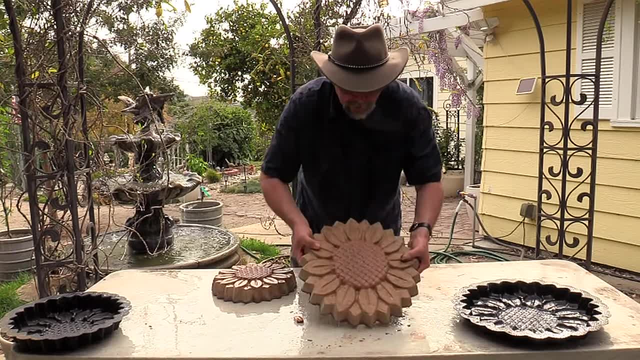 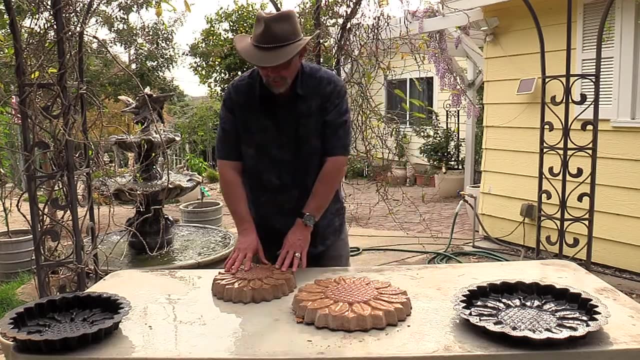 okay. so I just took these out of the mold- very easy to do. i let them down, you know, to get the some of the dust off. you can see that you've got your brown and your buff, both of them looking really good. um, the colors are nice and subtle and pronounced. the buff has enough yellow into it that we get the symbolism behind it.